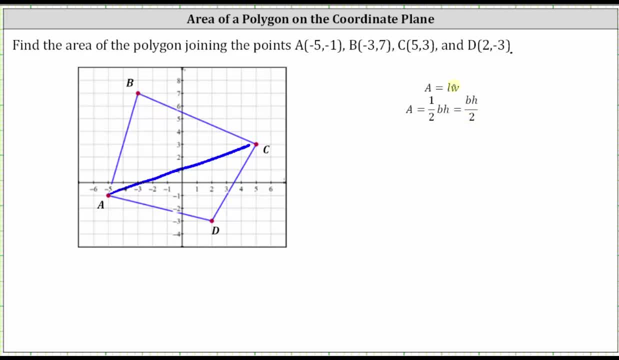 or base times, height divided by two. So in this case, I think it's going to be better to think outside the box. In this case, think outside the given quadrilateral. Let's inscribe the quadrilateral in a larger rectangle. To do this, the left side of the rectangle. 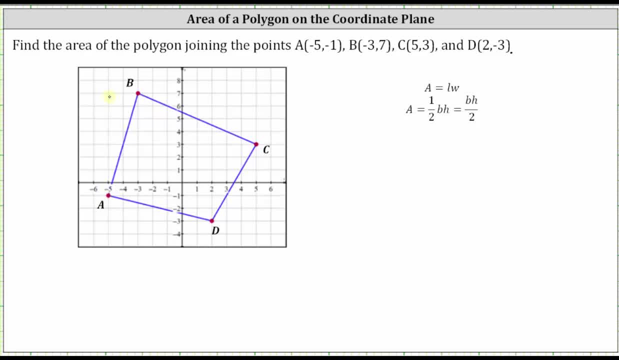 must include point A, go as high as point B and as low as point D, and would look like this: The side on the right must include point C and look like this: The side along the bottom must include point D and the side along the top must include point B. 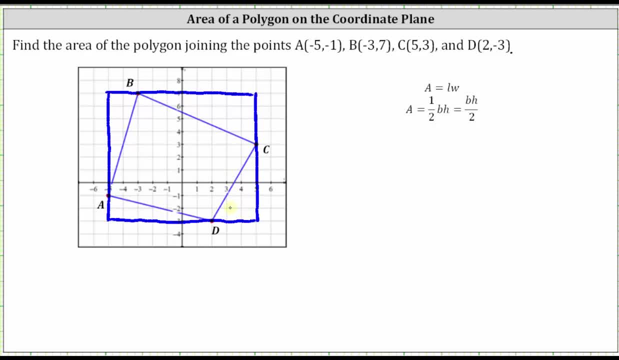 Because of the way it's situated on the coordinate plane. we can easily determine the area of the circumscribing rectangle using the formula length times width. Let's go ahead and find the dimensions of the larger rectangle. Notice how the bottom side is parallel to the x-axis. 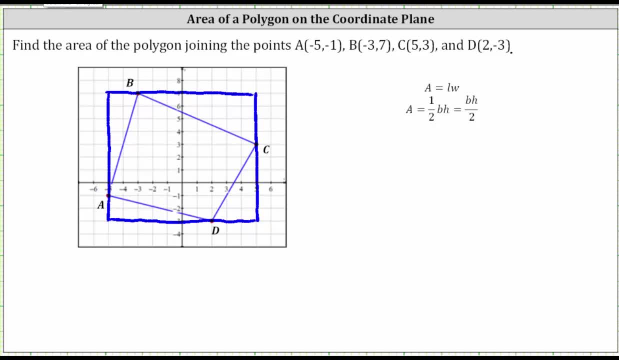 where the values go from negative five to positive five and therefore the length is 10.. Of course, we could also count the units along the side to verify it is 10 units, And then for the length on the right side, notice how this side is parallel to the y-axis. 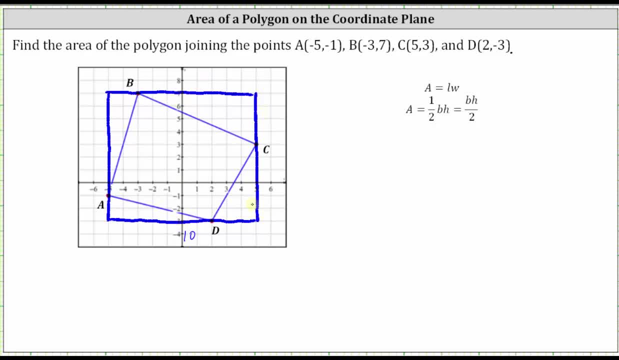 where the values go from negative three to positive seven, and the length on the right is also 10.. So in this case we actually have a square that is circumscribing the given quadrilateral. From here, notice how, if we find the area, 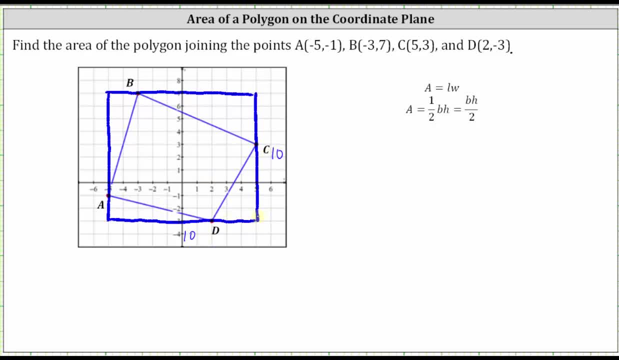 of the circumscribing square. it will be too much area. So from here, if we subtract out the areas of the right triangles formed at the corners of the circumscribing square, the remaining area will be the area of the original quadrilateral. 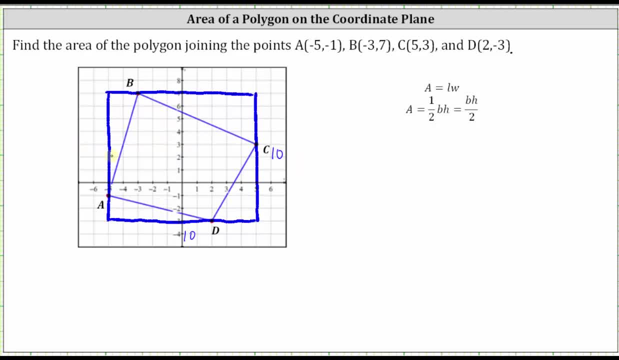 meaning, once we find the area of the larger square, we will subtract out the area of this right triangle, this right triangle, this right triangle and, finally, this right triangle. The area that's left will be the area of the given quadrilateral. 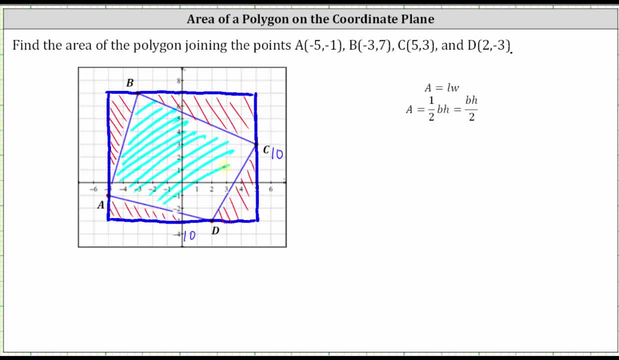 shaded here in light blue, And it'll be easy to find the base and the height of the right triangles because of the way they're situated on the coordinate plane And because we have right triangles, we use the length of the two legs for the base and the height. 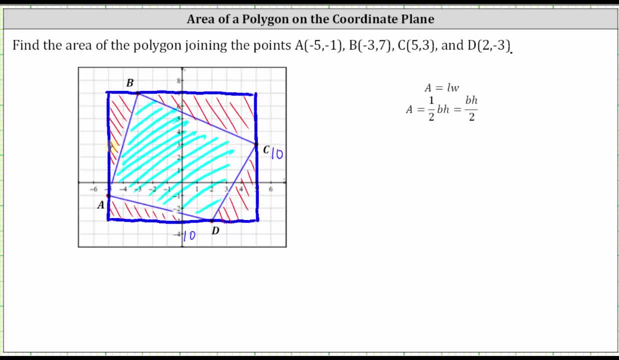 Let's go ahead and find those lengths. now For the triangle in the upper left-hand corner, notice how the short leg has a length of two units. The longer leg has a length of eight units. In the upper right-hand corner, the shorter leg has a length of four units. 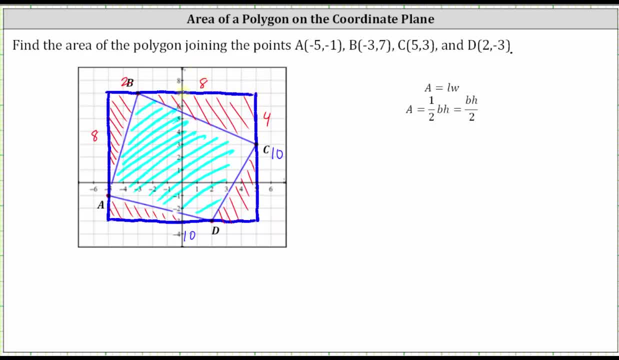 The longer leg has a length of eight units. Remember, we know the length of the entire side of the square is 10 units. Notice, two plus eight, Eight is 10.. And now for the right triangle in the lower right-hand corner. 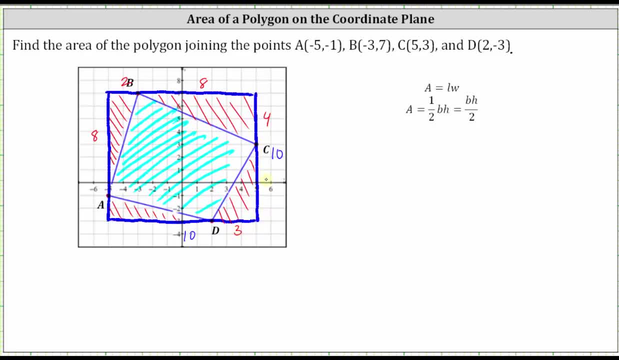 the short leg has a length of three units. The long leg has a length of six units. Notice: four plus six is 10.. And then, finally, for the right triangle in the lower left-hand corner, the short leg is two units. Two plus eight is 10.. 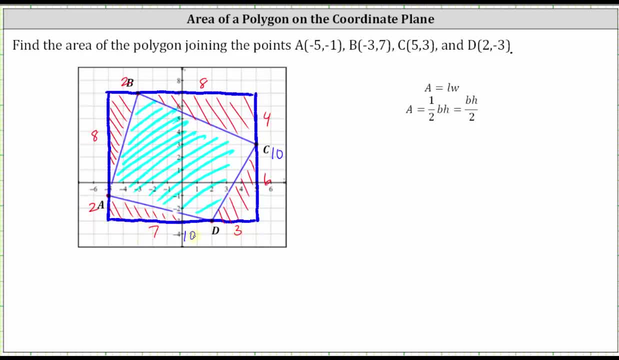 The longer leg has a length of seven units. Seven plus three is 10.. So now we have all the dimensions that we need to find the area of the polygon formed using points A, B, C and D. Our formula is going to be the area of the quadrilateral. 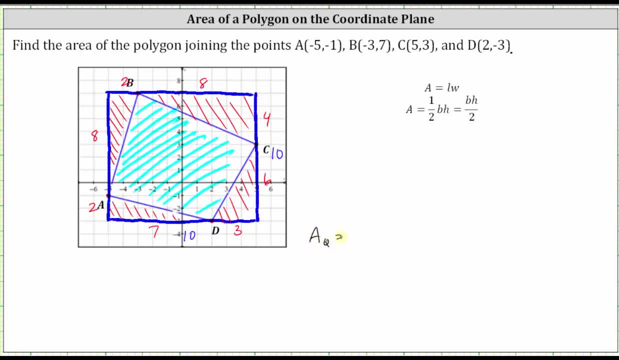 A sub Q is equal to the area of the circumscribing square, which we'll call A sub S, and then minus the sum of the areas of the four red right triangles, which we'll call A sub T sub one, plus A sub T sub two. 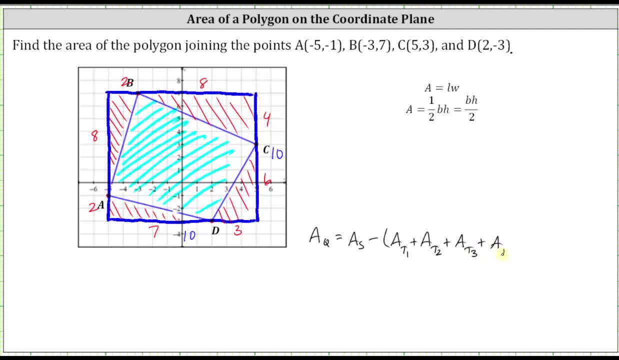 plus A sub T sub three, plus A sub T sub four, And now let's find all of these areas. So again, A sub Q, the area of the quadrilateral is equal to the area of the circumscribing square, which is 10 times 10,. 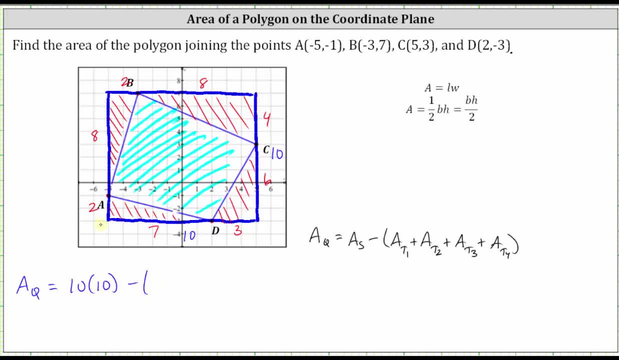 and then minus the sum of the areas of the four red right triangles. Starting in the upper left-hand corner, the area of the right triangle is equal to one half times eight times two. Remember we used the two legs as the base and the height. 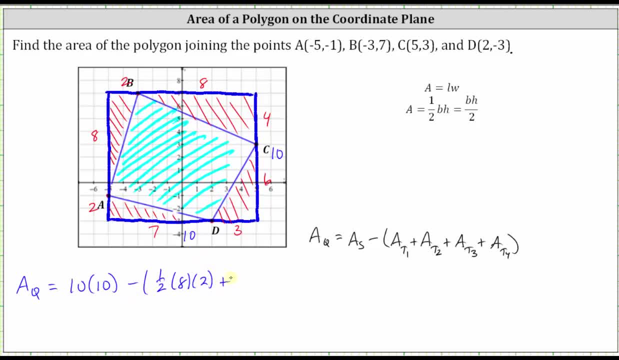 and the order doesn't matter. Plus, moving clockwise, the area of the right triangle in the upper right-hand corner is one half times eight times four, plus the area of the right triangle in the lower right-hand corner, which is one half times three times six.